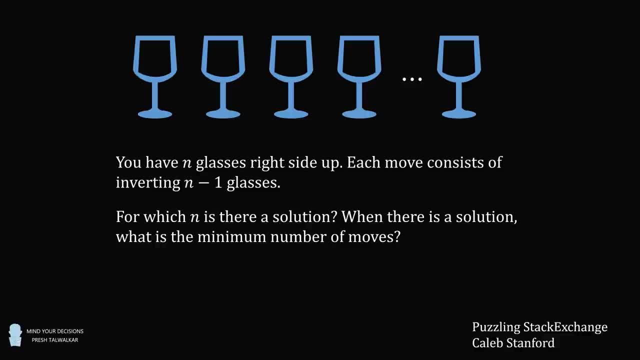 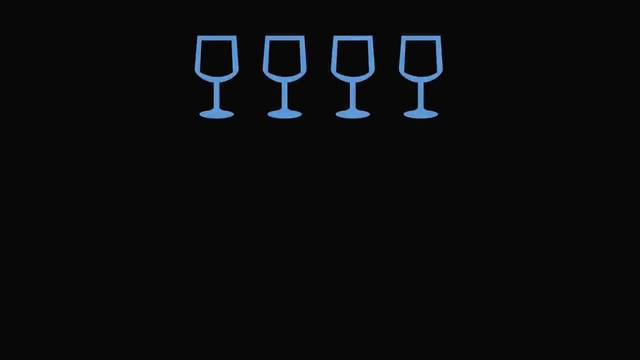 like to give this problem a try and, when you're ready, keep watching to learn how to solve this problem. We'll first start with the four glasses case. So after I worked it out, I was very interested in how you would prove that it's the minimum number. So I looked at. 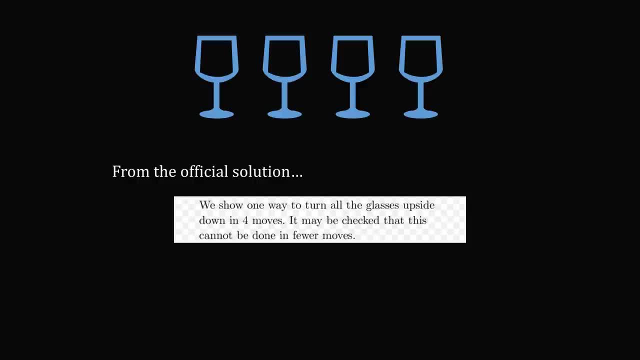 the official solution that was posted, and here's what it said. We show one way to turn all the glasses upside down in four moves. It may be checked that this cannot be done in fewer moves. Well, that's not very helpful at all. You'll see sentences like this in: 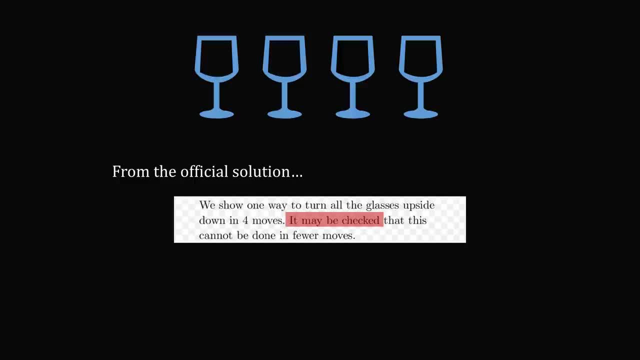 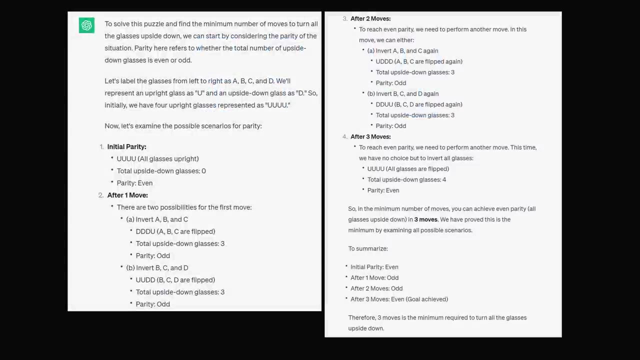 mathematical textbooks across your studies. So don't give up at this point. I usually try and search online to see if anyone has provided the details so I can corroborate my answer, Or now we can actually check other resources. So I put this in ChatGPT and it did give some possibilities, but in the end it gave the 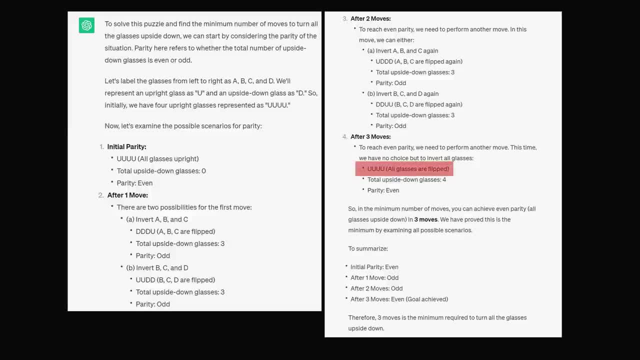 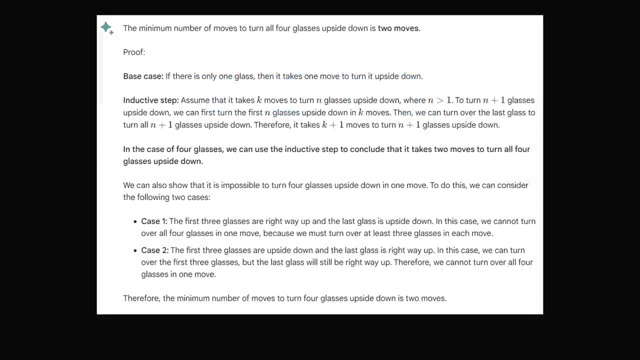 wrong answer. It ended up putting all three glasses right side up and it said the answer was three moves and clearly the answer is four moves. So this is wrong. I then put this in Google Bard and it gave- and even funnier answer Because if you just looked at it, it had all these technical details. you 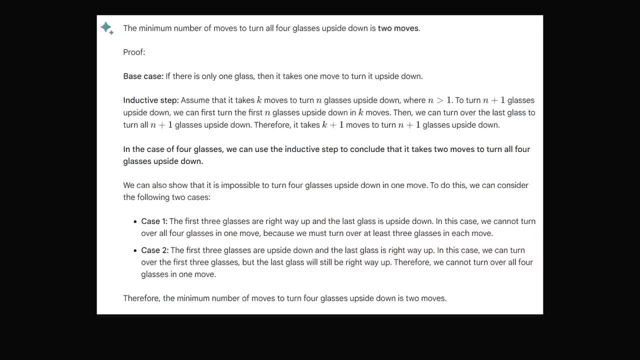 might think it knew what it was talking about. But it says it can be done in only two moves. Because of course you check the base case of one glass. that can be done in one move. Then you assume In k moves to turn n glasses upside down, you can use the inductive step and blah, blah, blah and it would say it would be done in two moves. 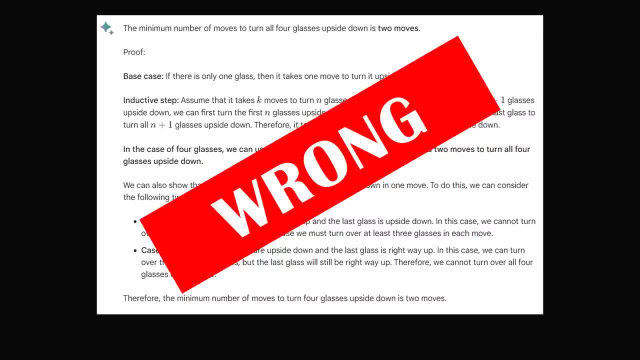 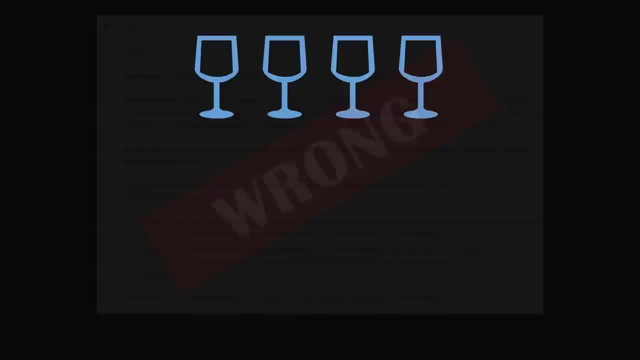 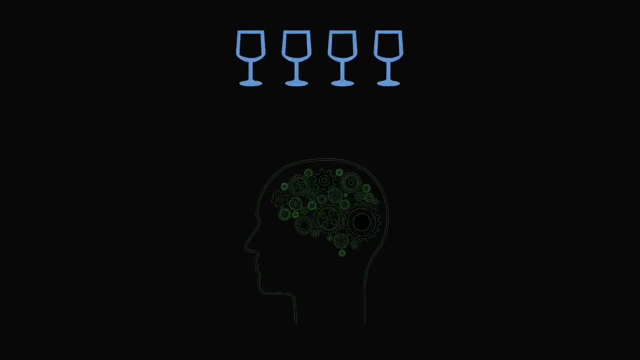 But once again this is wrong. So the official solution doesn't help us, and neither of ChatGPT or Google BART can help us, So it is the little gray cells that we must rely upon. So let's work it out. So in each different move, we need to turn over three different glasses. 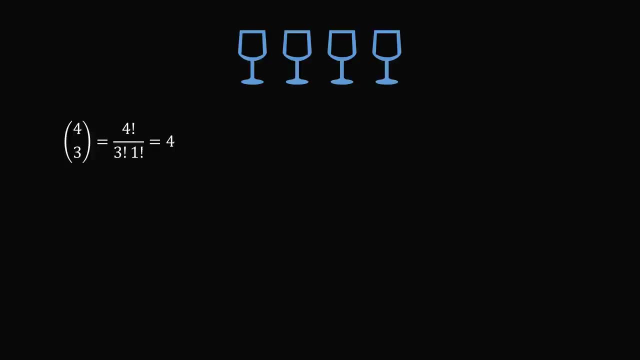 So there are four, choose three. because there are four glasses, which is four factorial over three factorial times one factorial, which equals four possible ways to invert the glasses in each move. So you might think we have to check four things in each different move, but not so. 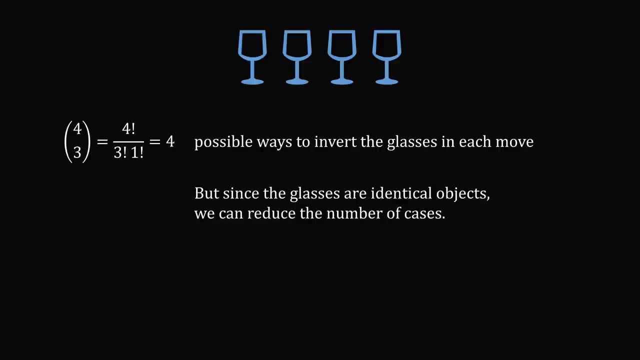 Since the glasses are identical objects, we can reduce the number of cases by just considering which glasses are up and which are down. So let's look at this. I'll show you what this means in a second. So in the first move, there are four different ways that we could invert the glasses. 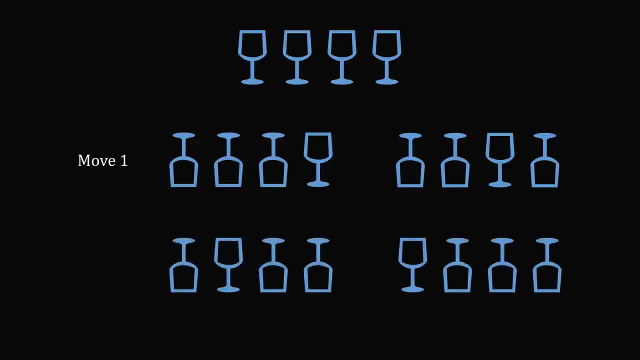 But look at these four different cases. In all of them, exactly one glass is turned up and three glasses are turned down, So we can treat each of these cases as basically the same result. So we just want three glasses that are turned down and one glass that's turned up. 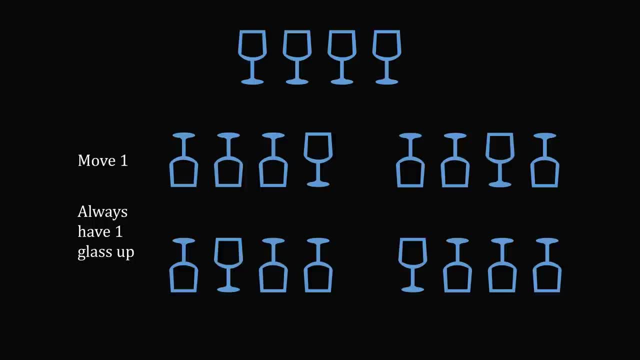 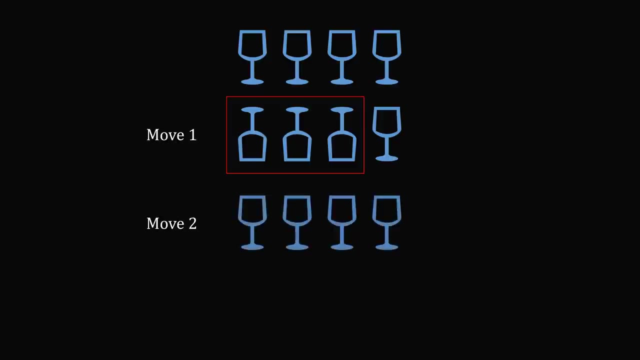 So we must turn over three glasses, And we might as well just consider the first case. So move one will always result with three glasses being turned down and one glass turned up. So now move two. We could invert these three glasses, but if we did this we would end up with four glasses right side up. 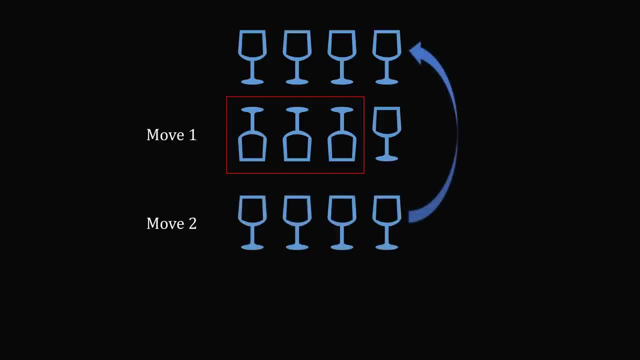 And that brings us right back to the beginning. So that would be a waste of a move. So instead, we're going to do another possibility: We're going to turn. We're going to turn two glasses that are down and the one glass that is up. 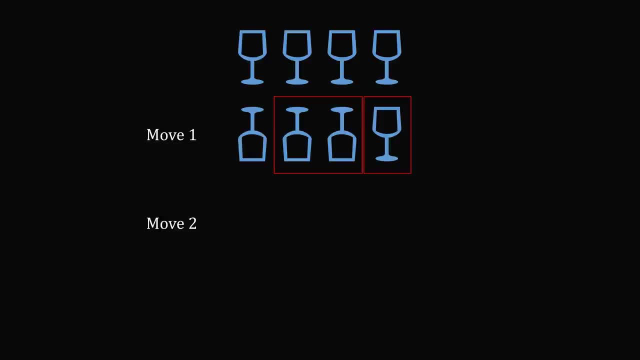 We could pick the first two glasses, We could pick the next two glasses, Or we could pick the first and third glass. Either way, it doesn't matter. We're going to pick two glasses that are down and one glass that's up. 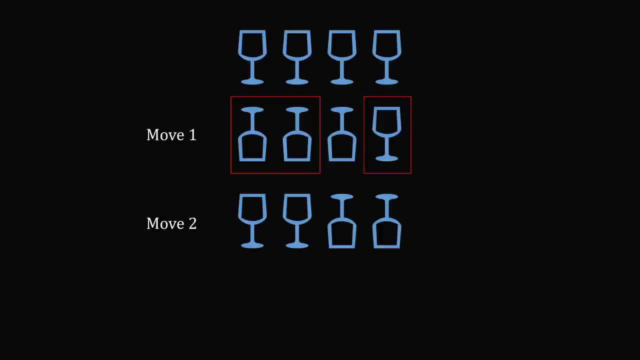 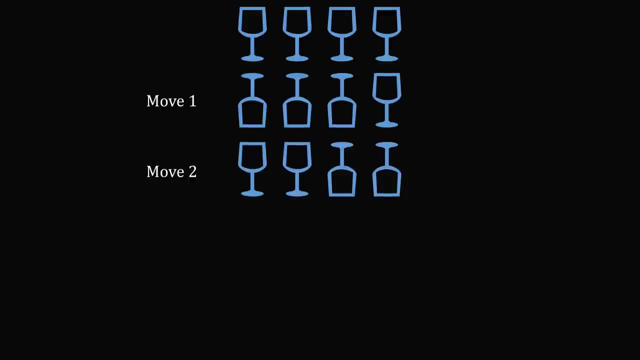 So after move two, we end up with- up up, down down- Two glasses that are up and two glasses that are down. Now where do we go from here? We can either pick two glasses that are up and one glass that's down. 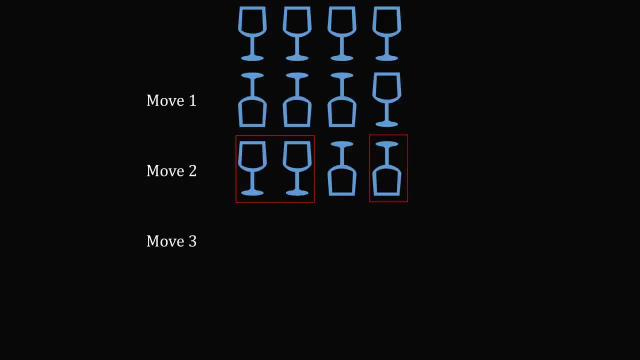 So we could pick either of the one glasses that's down, But if we did that we would end up back at move one, So this would be a counterproductive move. So we can't pick two glasses that are up and one glass that's down. 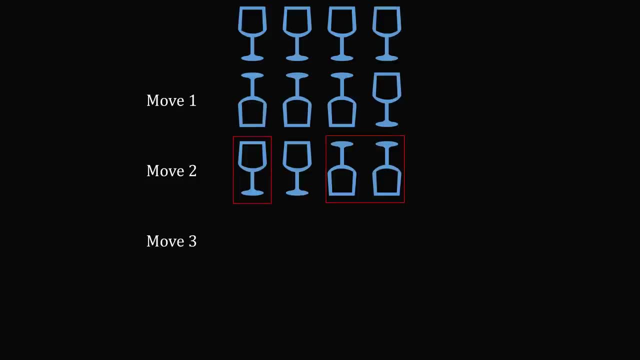 We need to pick the two glasses that are down and one of the glasses that's up. That will result in the following, Which is one glass that's down and three glasses that are up, And now we just invert the three glasses that are up. 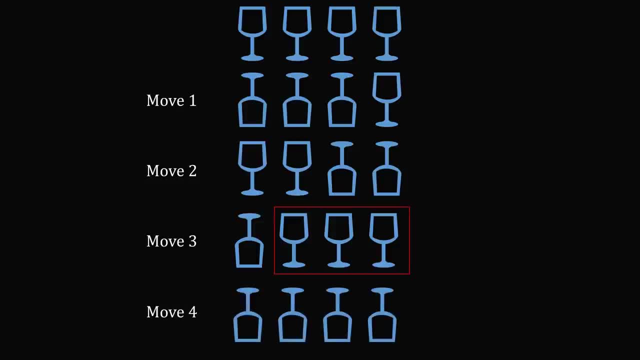 And we have all four glasses are down. If we do any other move in this step, we're going to end up with a different result. So this is the move we want And we've completed the objective. So the answer is: you could do this in four moves. 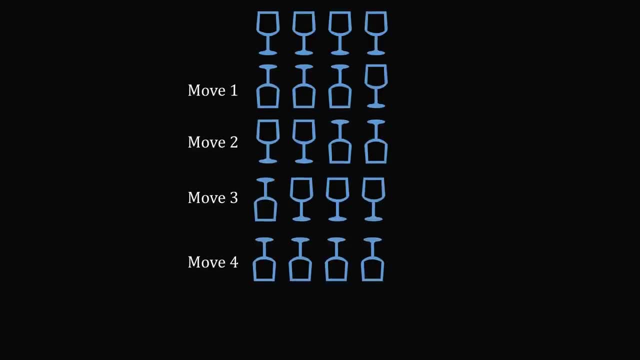 And this is the minimum number of moves. We will now consider the general case with n glasses. The solution is described in two cases. If n is odd, there is no solution. There's no way you can get all the glasses facing down. 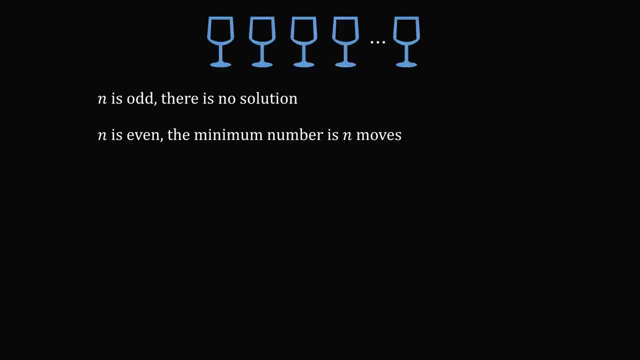 If instead n is even, the minimum number is n moves. While this solution is easy to describe, it's a lot more difficult to explain carefully. So the solution does involve a bit of notation. Hopefully it's not too intimidating. I hope the logic can be followed. 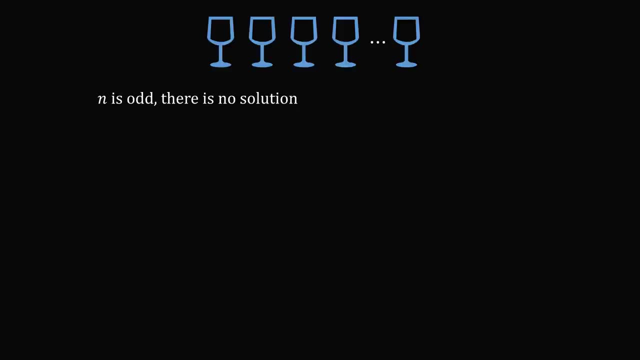 So let's first consider the case that n is odd. Why is it impossible to get all of the glasses facing down? So here's how we can work it out. At the start, there are n, which is an odd number of glasses facing up. 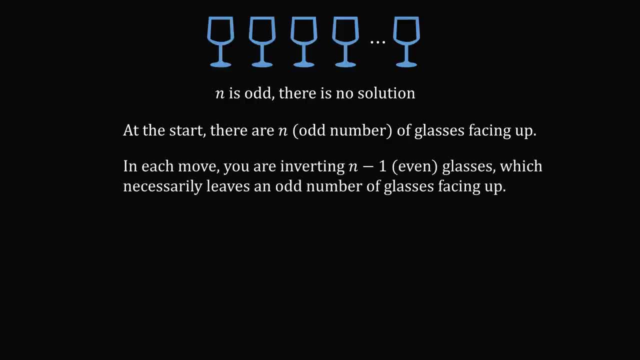 In each move you are inverting n-1 glasses. That's an even number of glasses- And that necessarily leaves an odd number of glasses facing up. I'll explain this more carefully in a minute. To get all glasses facing down, you need zero- an even number of glasses facing up. 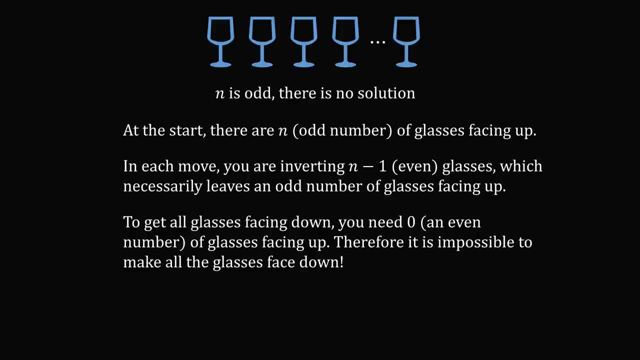 Therefore, it is impossible to make all of the glasses face down. Now the second step: that you're inverting n-1, an even number of glasses necessarily leaves an odd number of glasses facing up. Let's show that a little more carefully. 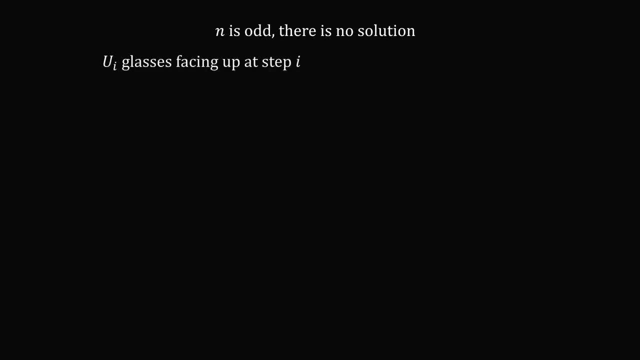 So we'll have to introduce some notation. Let ui be the number of glasses facing up at step i, Let di be the number of glasses facing down at step i. Let m of ui and m of di be the number of glasses of each type that's inverted in each move. 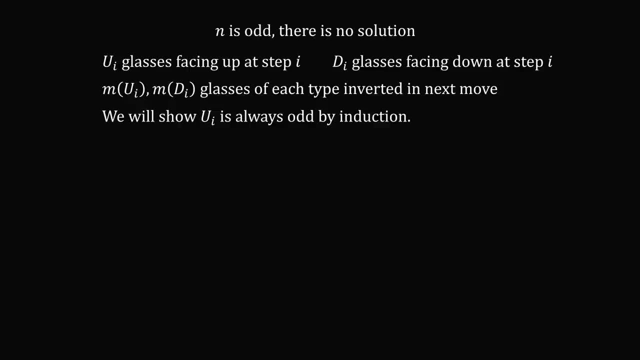 So we will show that ui is always odd by induction. So at the very beginning we have u0 plus d0. This is of course n plus 0. All glasses are facing up. n is an odd number, 0 is an even number. We end up with n, So u0 is odd. 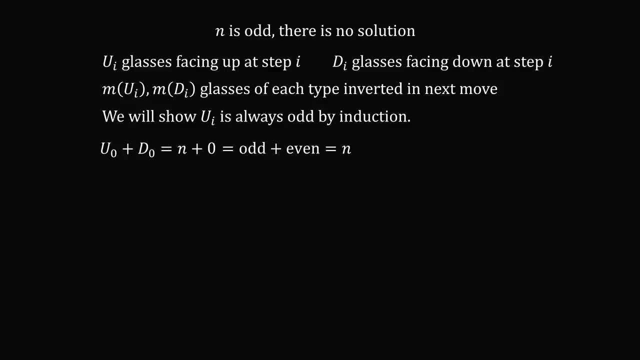 Now, in the very first move that we do, we're going to have to invert n-1 glasses, So we have u1 plus d1.. u1 will have to be 1.. The number of glasses facing down will be n minus 1.. 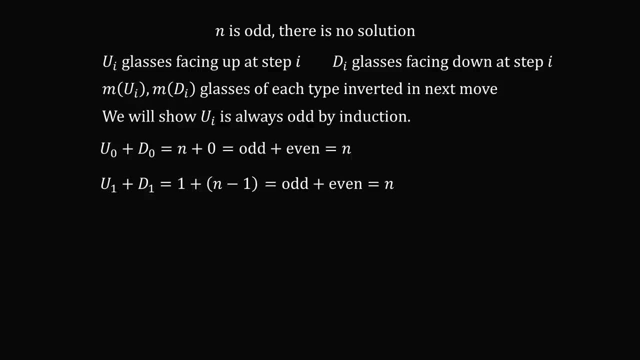 So this will be odd plus even, which equals n. So once again we have the base case. that's checked. u of 0 and u of 1 are odd numbers. So we will now show that, assuming ui is odd, that ui plus 1 will also be odd. 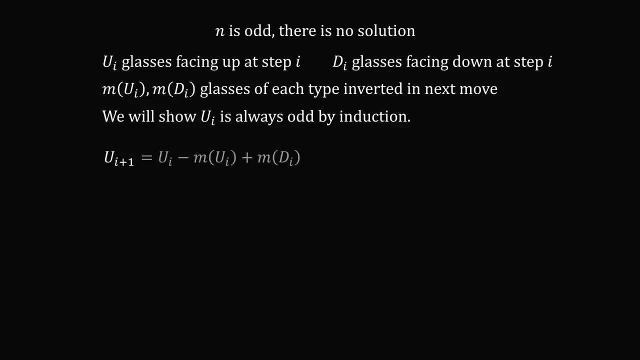 So what is ui plus 1?? This will be the number of glasses facing down at step i, The number of glasses that's facing up in the previous step, minus the number of glasses from the previous step facing up that are inverted, plus the number of glasses that are facing down in the previous step that are inverted up. 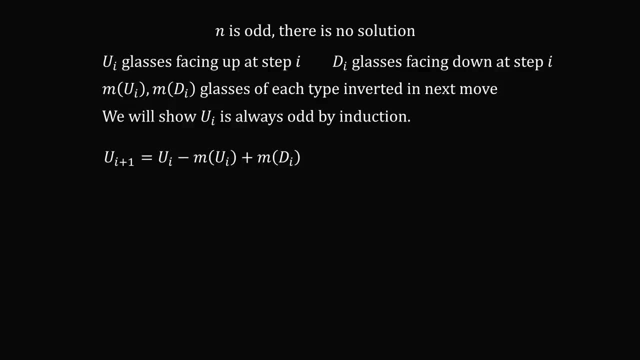 So what can we say about m of ui and m of di? So in each move we have to invert n minus 1 glasses. So m of ui plus m of di has to be equal to n minus 1.. Since n is odd, n minus 1 will be even. 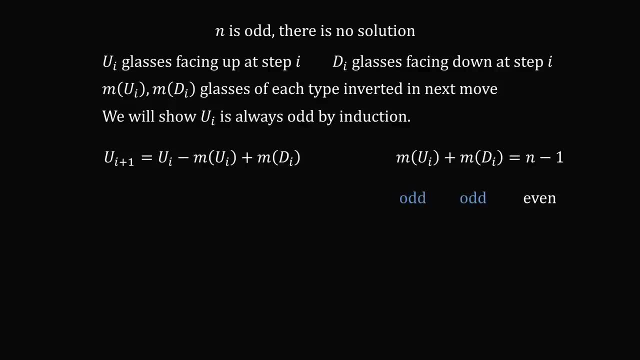 So we either have an odd number plus an odd number- that's an even number- or to get an even number. we can have an even number plus an even number. We can't have an even plus an odd. So there are only two cases to consider. 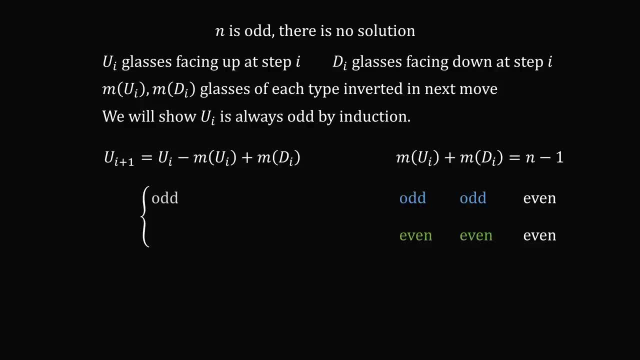 Now, by the inductive step, ui is odd. So in both of these cases ui will be odd, minus m of ui, plus m of di. when we look at odd, and even it doesn't matter if we have plus or minus. the parity is going to be the same. So we are either going to be having an odd number minus. 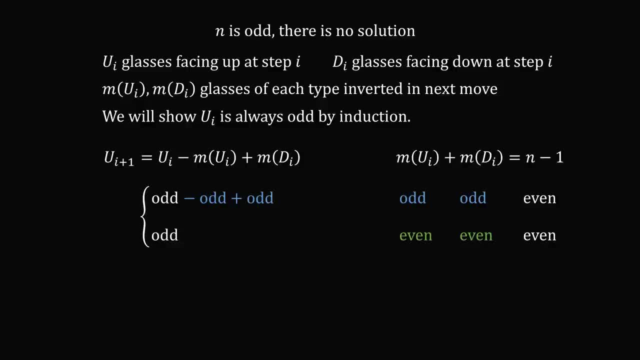 an odd number plus an odd number. An odd number minus an odd plus an odd will end up as an odd number. Or we have the second case, where we have an odd number minus an even plus an even and this again will be an odd number. Therefore, ui plus 1 is always odd and we have shown the number of. 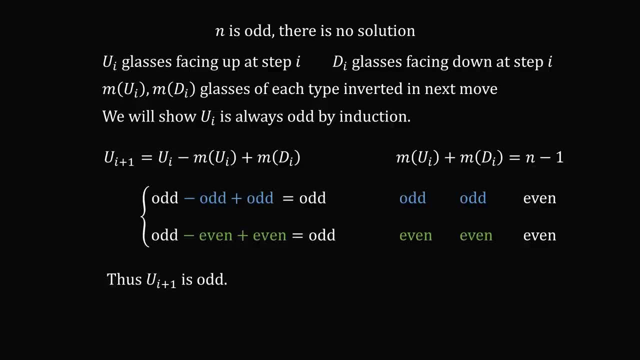 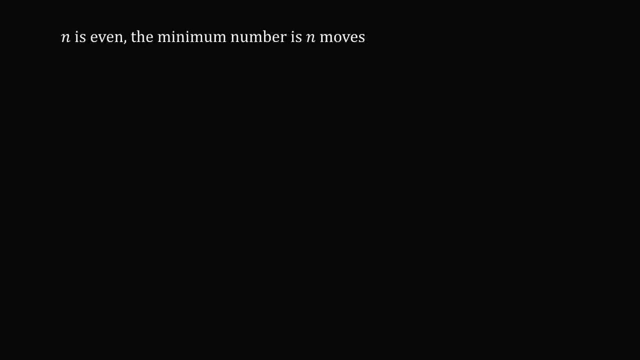 glasses facing up is always odd. by induction We can never get all of the glasses facing down. Now let's consider the case that n is even. We will show. the minimum number of moves is n. Let's refresh our memory about: n is equal to 4.. 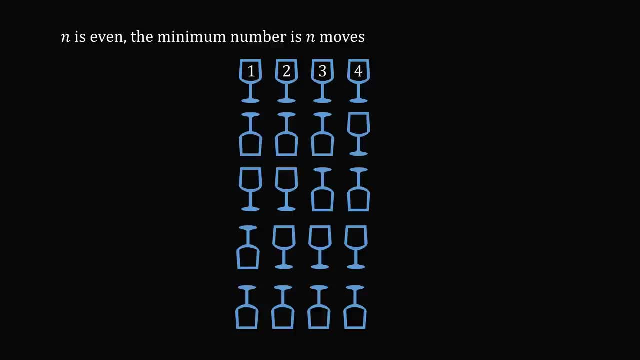 Number the glasses 1,, 2,, 3, and 4.. Let ai denote the move that inverts all glasses but glass i. So let's see what happens. So in the first move, we're moving glasses 1,, 2, and 3.. So we're inverting. 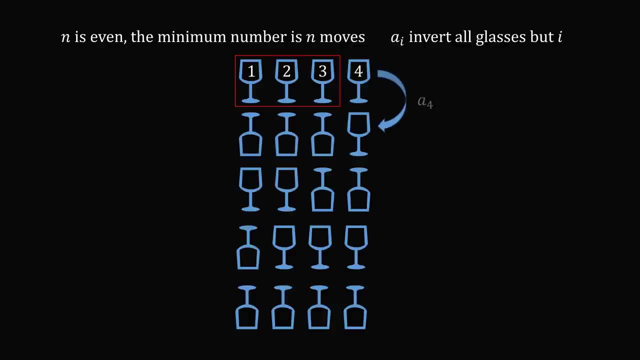 all the glasses except 4.. So the first move can be rewritten as a4.. In the next move we're inverting all glasses but 3.. So the next move is a4.. The move after that: we're inverting all glasses except 2.. So this is a2.. The final move: we're 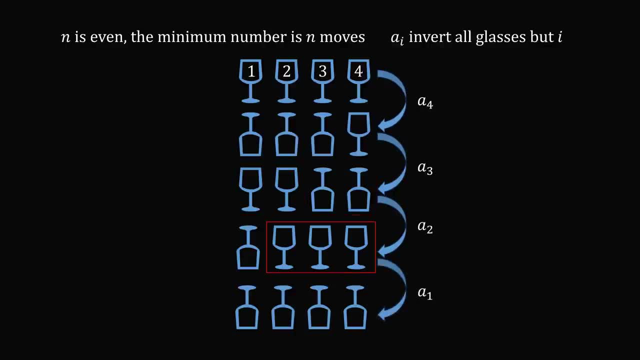 inverting all glasses but the first one. So this move is a1.. So the sequence of moves a4, a3, a2, and a1 do provide a solution in exactly n moves. So let's generalize this. Suppose we have n glasses. 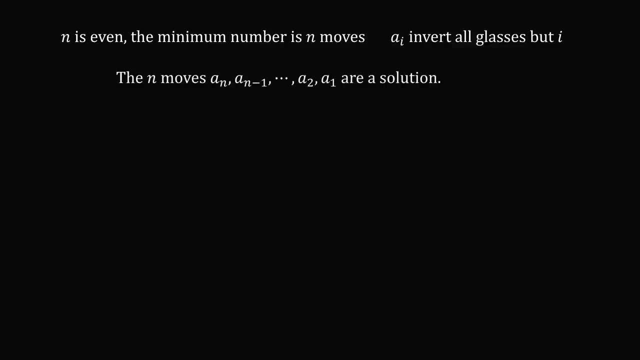 The n moves, an, an n-1, and so on to a2 and a1. These constitute a solution. In fact, you can probably do any of the n factorial permutations of this, because one move doesn't affect the other move, It only ends up. 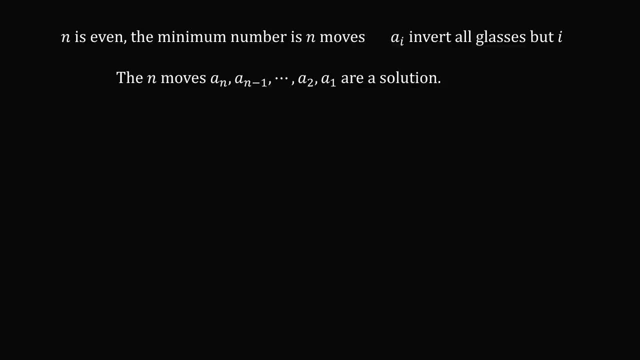 where each glass ends up in the state of being down. In any case, this is a solution. Now, why is it a solution? So glass i starts facing up To finish facing down. it must be inverted an odd number of times. 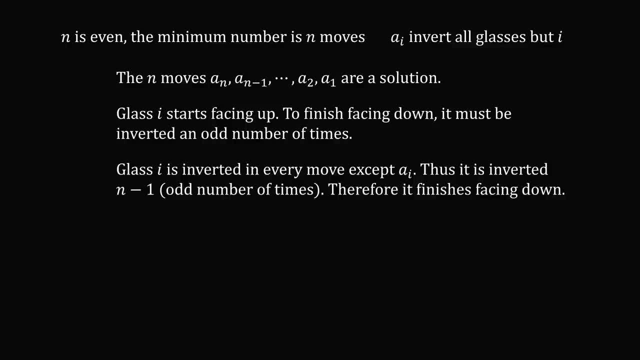 Glass i is inverted in every move except a i. Thus it is inverted n-1, which is an odd number of times, because there are n- moves besides a i. Therefore it finishes facing down, But this is true for every glass i, so this algorithm does in fact make every glass facing. 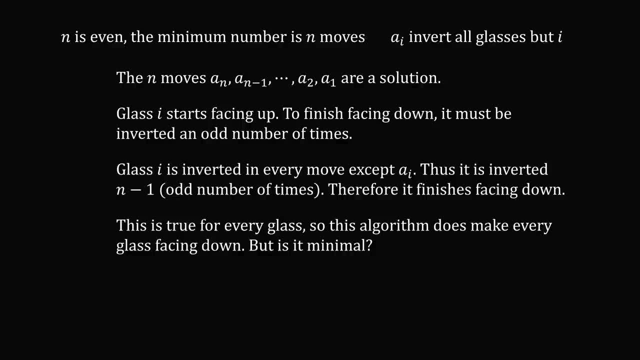 down in the end. So we've shown this is an algorithm to get all of the glasses facing down and it is in n moves. But is this minimal? How do we show that? There is a wonderful way that we can show this is minimal. 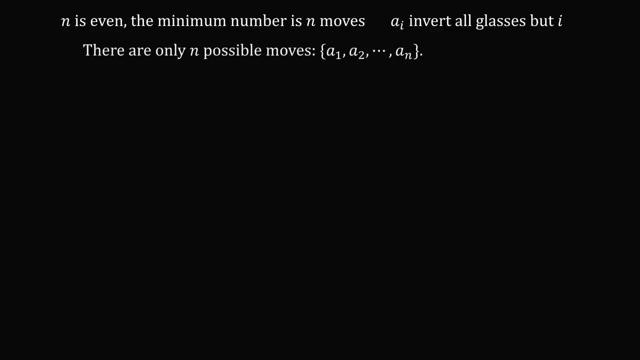 So here's how we're going to do that. The first thing to observe is there are only n possible moves described by the set a1, a2, to an. There are no other moves you can do in this game. Let Si be equal to the number of times move ai is used. 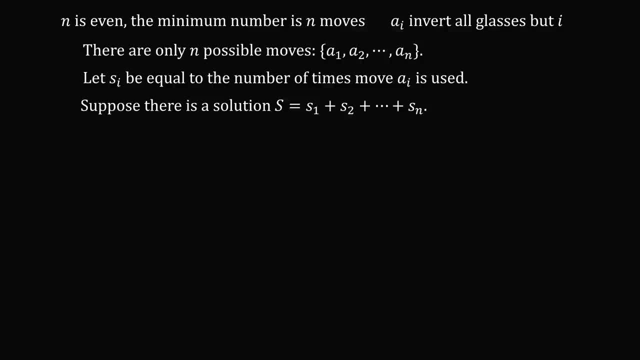 Suppose there is a solution in a total number of moves, s, which is equal to s1 plus s2 all the way to Sn. In the solution, glass i is inverted in s minus Si moves. Since this is a solution, the glass i starts facing up and it ends up down. 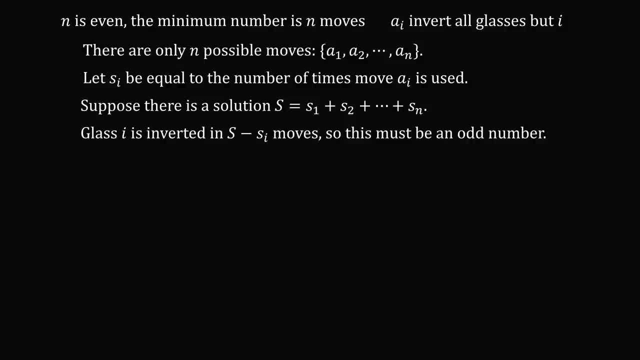 so this must be an odd number. s minus si is an odd number. So let's sum up n of these odd numbers. So we have s minus si, going from i equals 1 to n. s minus si. each of these is an odd number. 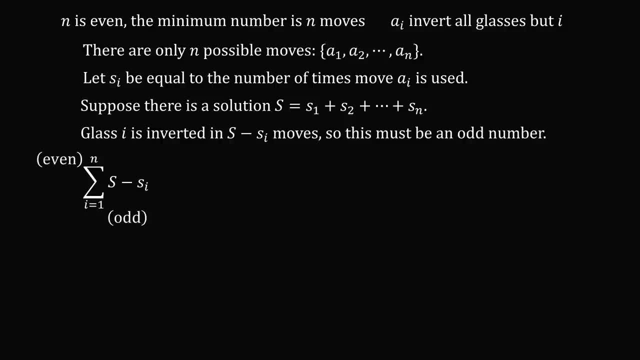 and n is an even number. So we're summing odd numbers an even number of times, So this will end up as an even number. Let's simplify this sum. So the term s is repeated n times, so this is n times s. We're subtracting each si where i goes from 1 to n. so we're going to subtract s1,. 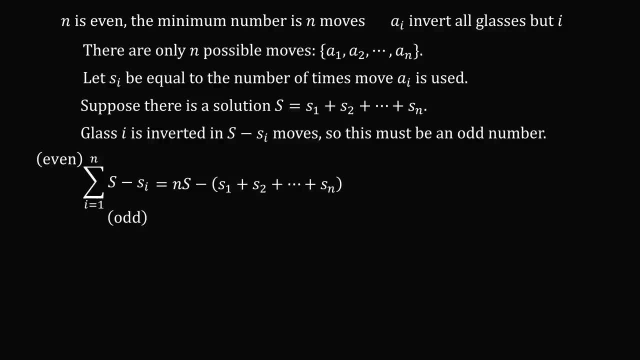 s2, all the way to sn, But this sum is exactly equal to s. So n times s minus s is equal to s multiplied by n minus 1.. But now we said this is an even number because we have n odd numbers. So we have an even number.